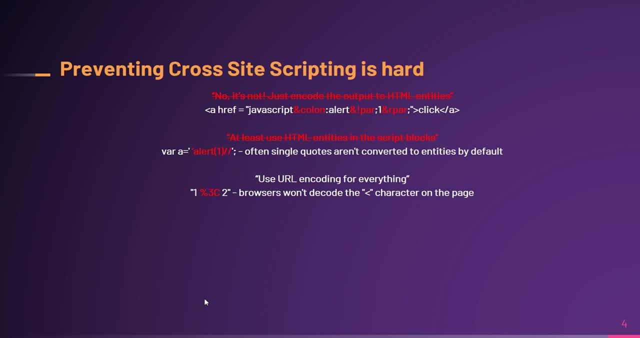 So if someone says that you use the URL encoding for everything, So the problem in this case is that the character You see here is so the browser won't be able to decode this particular character and it will only read like %3C. So all these methods won't work and somehow they may leave a loophole which will cause. 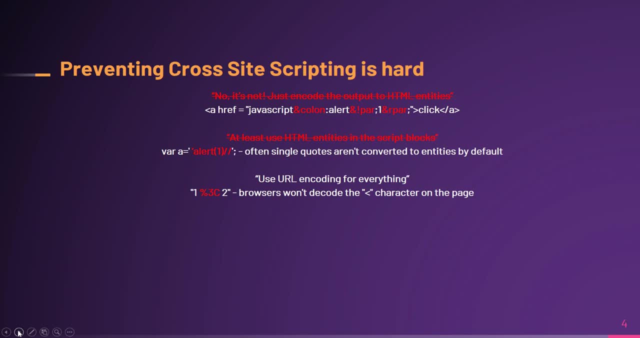 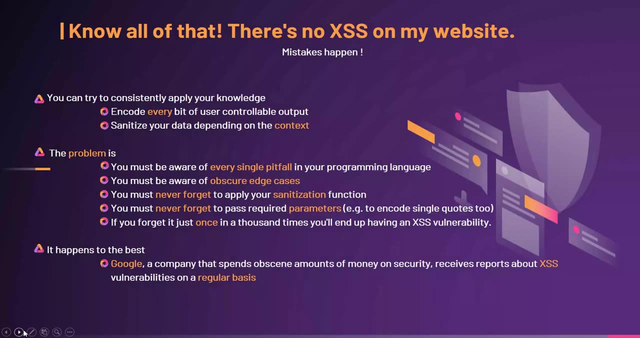 cross-site scripting and if you think that you can like block all the dangerous keywords, So this is not a good option. Now, now you know that, all so that there is no cross-site scripting on your website. You're sure about that, but there's some mistakes that can happen, So you can try to consistently. 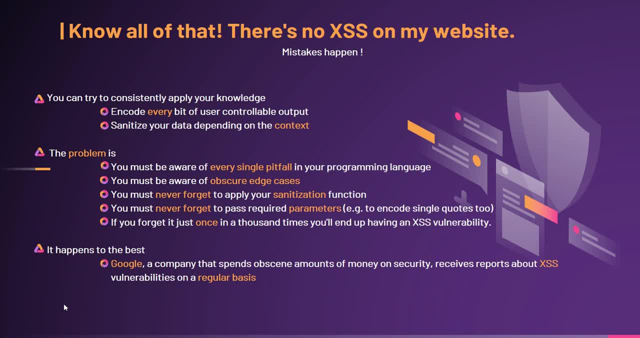 apply your knowledge. What you can do here is you can encode every bit of user controllable output and also you can sanitize your data depending on the context. But the main problem here is that you must be aware of There is no single pitfall in your programming language, and also you must be aware of obsecure. 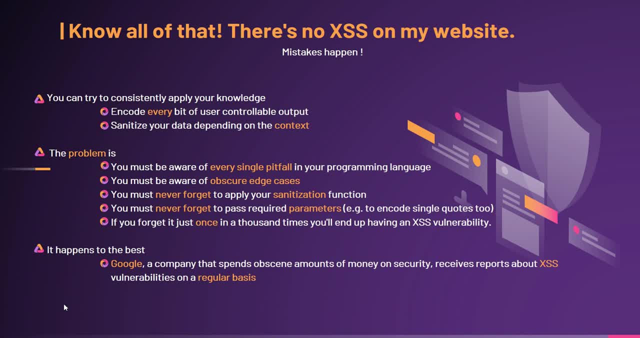 edge cases, and you must never forget to apply your sanitization function as well, as you must apply, or you must not forget to pass the required parameters. example, to encode single quotes too. If you forget it just just once in a thousand times, you will end up having an XSS vulnerability. 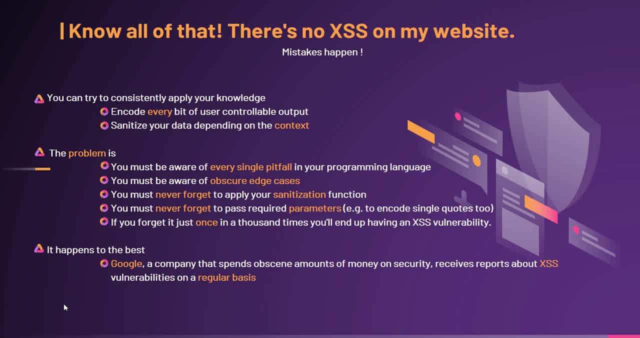 So if you are thinking that this vulnerability do not occur in like big companies like Google, Microsoft, Twitter and in all, then you're wrong, because they receives report about XSS vulnerability on a regular basis. even even if they spend a lot of amount on their security, they still get the cross-site scripting vulnerability on a regular basis on their website websites. 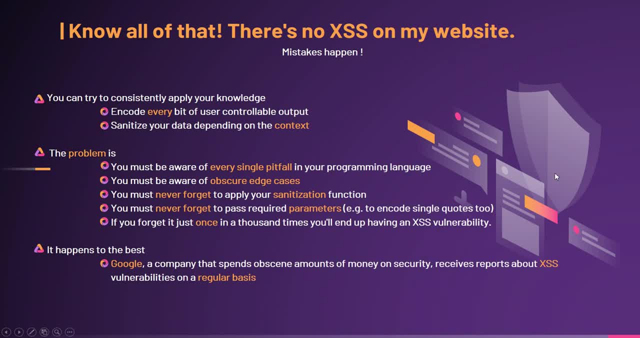 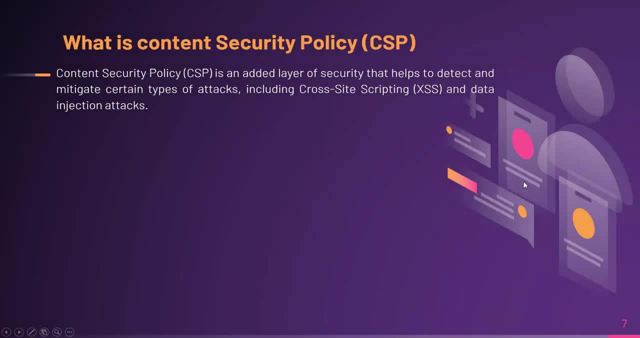 So this is some kind of attack which we cannot mitigate prop like a hundred percent, but we can do our best to mitigate it. So in order to add a layer to of security to the cross-site scripting attack, we use the content security policy header and it also prevent the data injection attacks that. 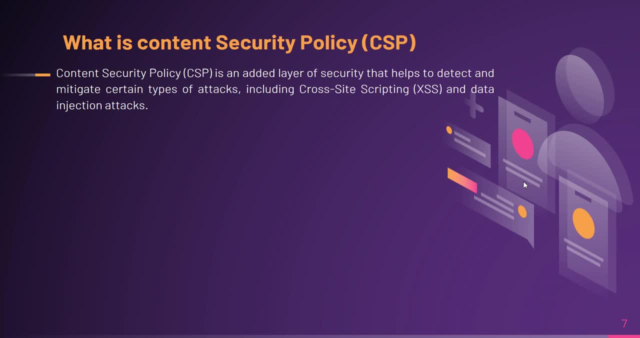 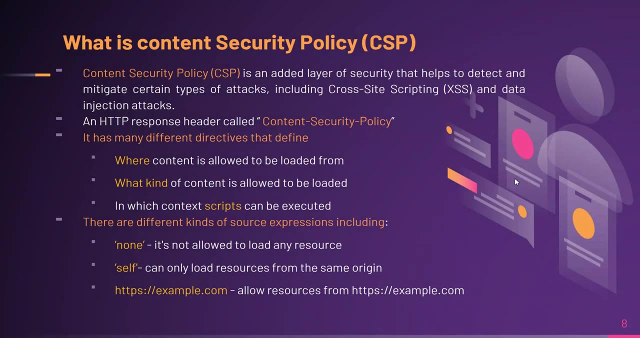 can happen to a particular website. So basically this is a Related to the Response response of the particular application. So you can also say that an HTTP response header can call content security policy. Now in the content security policy header you will see directives and each director. 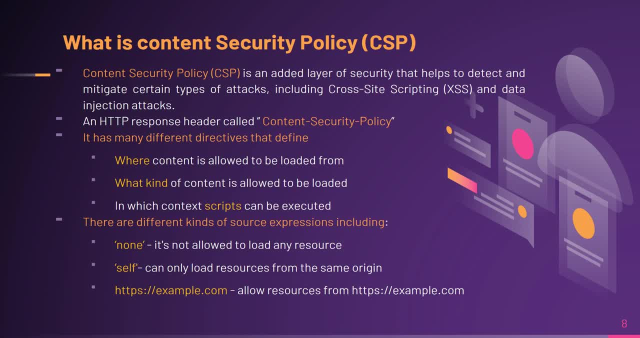 will have their source expressions. What I mean by this, I will Explain it in the later slides. So for the directives where content is allowed it to be loaded from. So it will tell you from where you can like load the content and what kind of content. 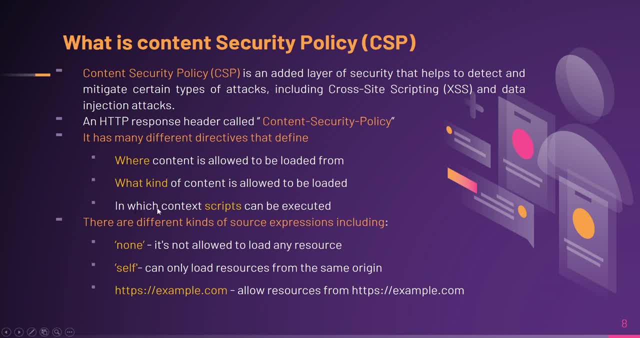 is allowed it to be loaded and in which context scripts can be executed. So for the director- we have to make sure that we remember these three points- and for the source expressions. So for the source: First is none, second is self and third is example dot com. so when you set the source, 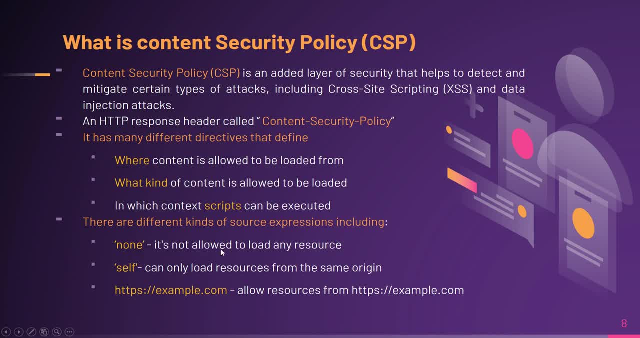 expression to none, It's not allowed it to load any resource. it will not load and resource into your application when you set it to self. it will only load the content from the same origin. And in the third case, when you set a particular define a resource. 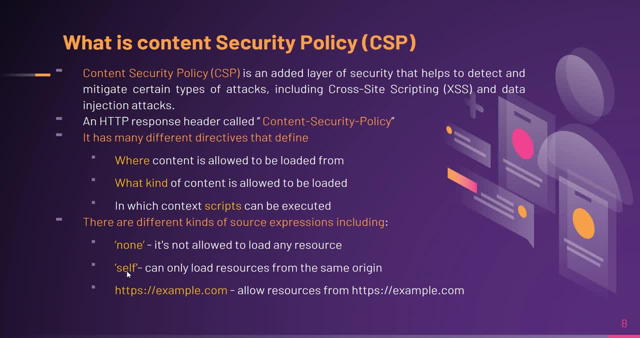 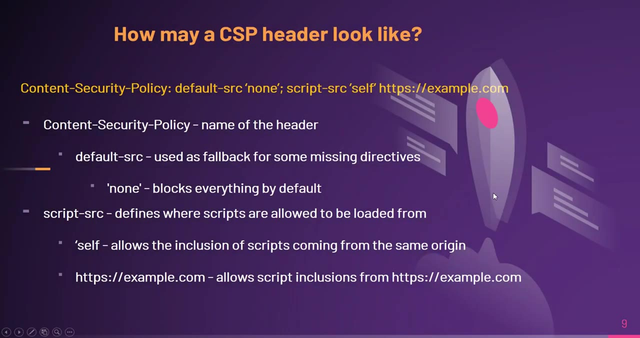 Like A region or a domain, a particular domain, like HTTPS, example dot com, then it will only allow the content or data from the resources from the example dot com. So let's move ahead. So how may a CSP header look like? So this is a CSP header. 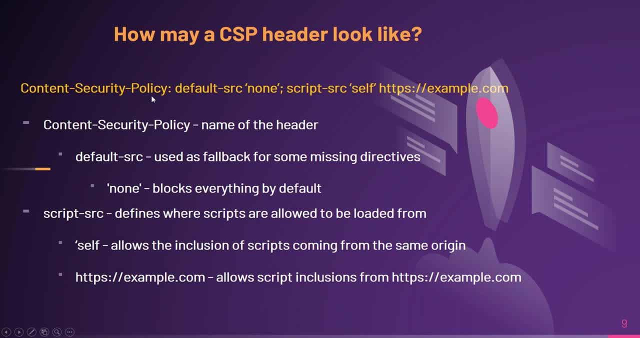 Now tell you that how and what it means. So First, As you can see that, CSP security policy- This is the name of the header. This is just a name of the header, And then, after that, the default SRC. It is used as fallback for some missing directives. 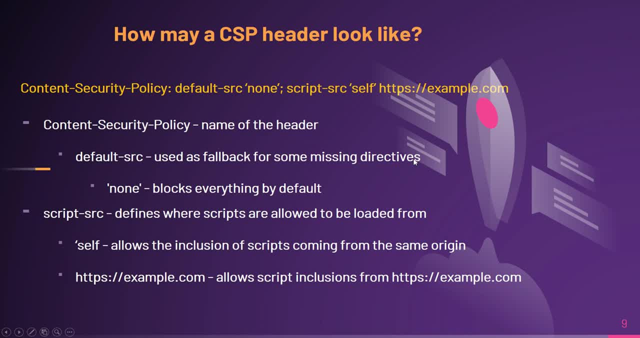 So, like you cannot the directives that you don't need in your particular CSP policy, You can use the default source and it set its value to none. then what none will do, it will block By default, And these are directives. default source and script source are directives. 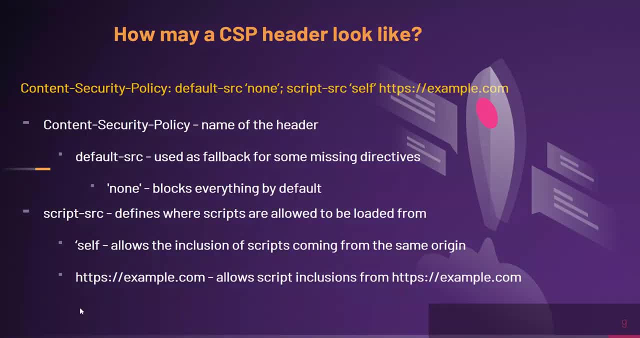 And when you say about none, So none is this. source expressions. Now, next directive is source script, So it will define from where scripts are allowed to be loaded from and source expressions is set to self and HTTPS, example: Dot com. So what this mean here? we want the scripts to be allowed it from the same origin. 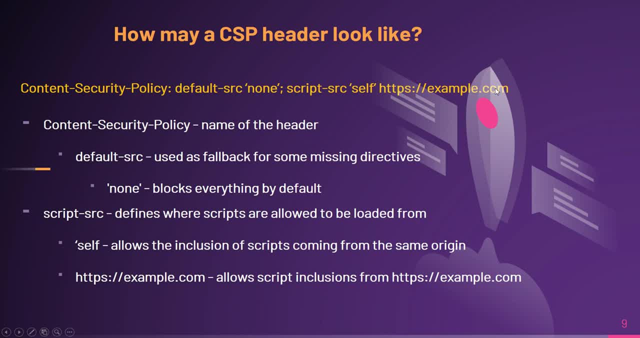 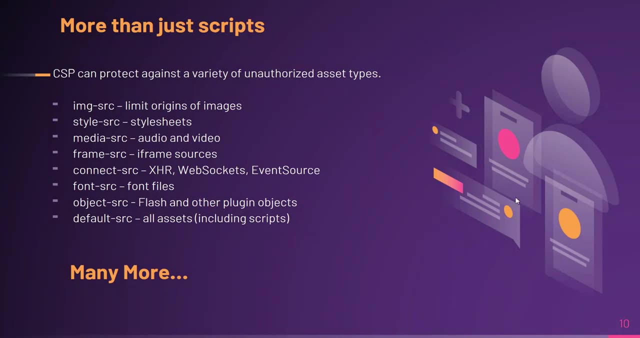 And we want the resources to be. we want the scripts to be loaded from, example, dot com. So this particular header means this. Now, in your particular header, you can add these directives, which are: image source, style source, media source, frame source, connect source, front source, object source, default. 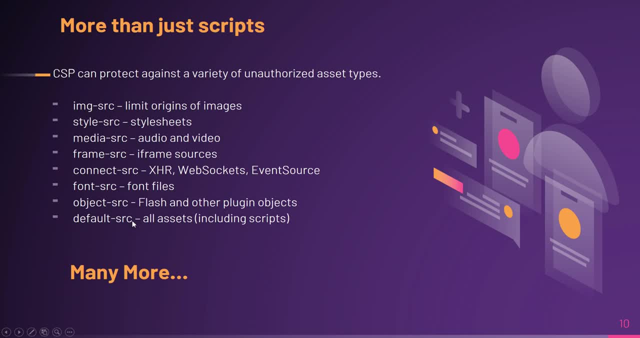 source. So each directive is used for different, different requirement. Let's say you want the media source and you want the audio and video to be loaded from a particular source, So you will use this media source. If you want your media source to be set to self, then it will load the resources from. 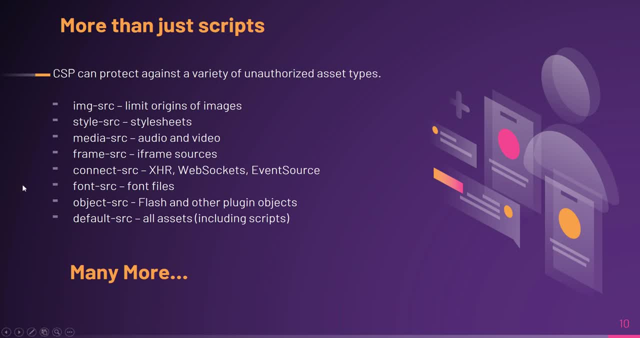 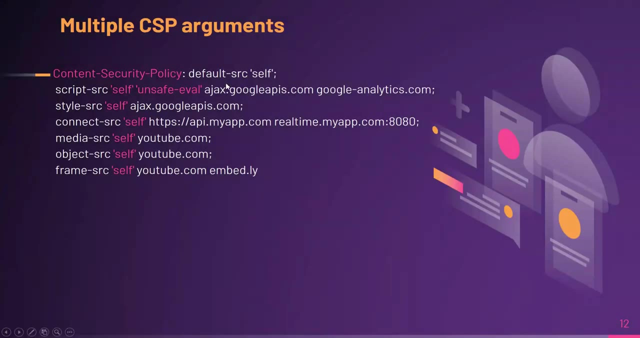 the same origin. OK, Same goes for the front source and each directive. you can define their particular like expressions. So let's move ahead and let's see. So in this example, what we see here is that content security policy, the first default source, is set to self.